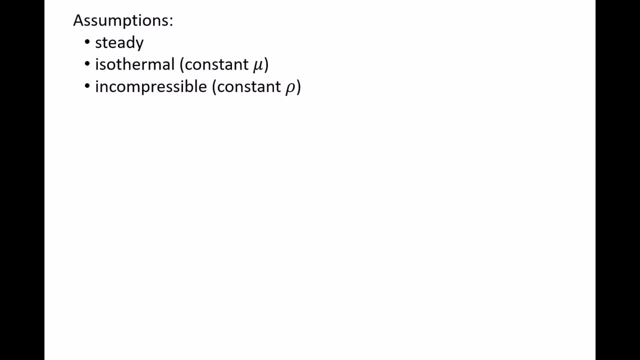 typically encountered in many pipe networks. We first examine pipes in series. Here we have three pipes with three different diameters: D1,D2, and D3.. The flow enters at point A and exits at point B on the right. Since the flow is steady through the pipes, the mass flow rate. 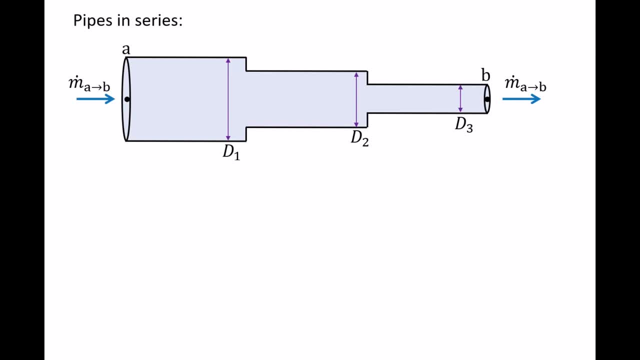 from A to B, which is denoted as m dot AB, is the same throughout the three pipes, That is, m dot AB is equal to m dot 1, is equal to m dot 2 and equal to m dot 3.. Since the mass flow rate is equal to the density rho times the volumetric flow rate, Q. 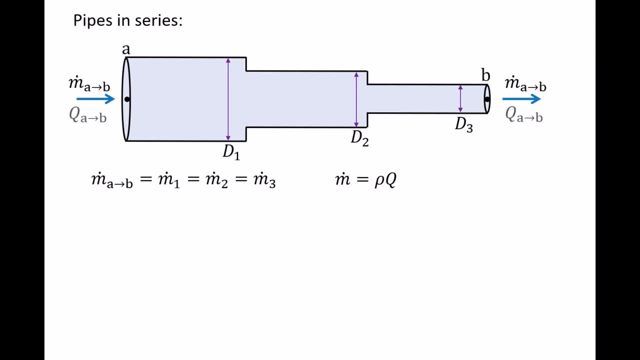 and the density is constant. this means the volumetric flow rate is constant throughout the three pipes as well, and we will call this flow rate QAB. So QAB is equal to Q1 and equal to Q2 and equal to Q3.. From now on, we will usually: 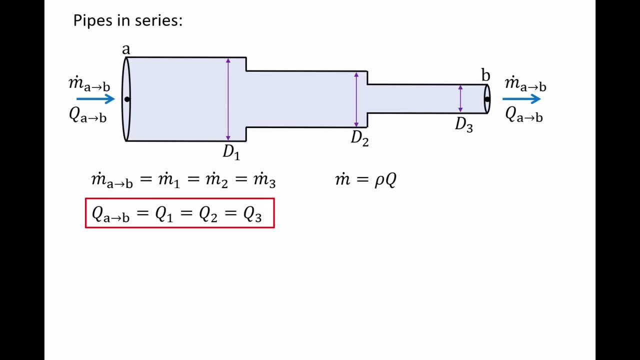 use volumetric flow rates rather than mass flow rates when using conservation of mass. The volumetric flow rate is equal to the flow speed v times the cross-sectional area A, And since the pipe diameter changes, the speed changes as well to maintain a constant volumetric flow rate. 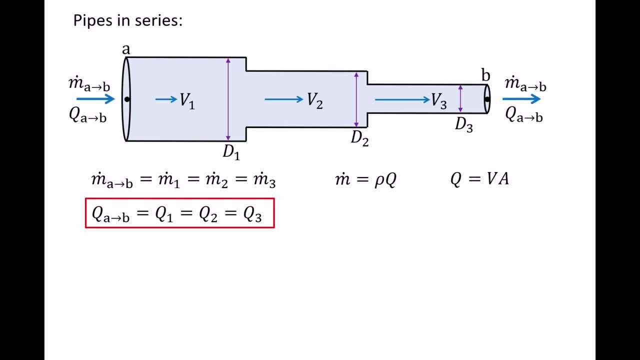 Now let's apply the conservation of energy equation from point A to point B. We draw a control volume around the three pipes denoted by the red dashed line, with an inlet at A and an outlet at B. The conservation of energy equation is the pressure head plus velocity head plus elevation. 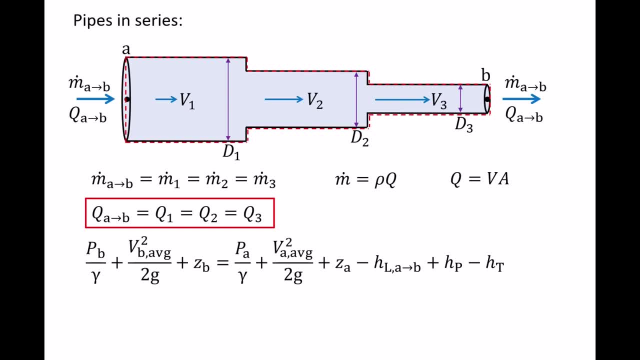 head plus velocity head plus elevation head plus elevation head plus velocity head plus elevation head at outlet B is equal to the pressure head plus velocity head plus elevation head at inlet A, minus the head loss from the inlet to the outlet plus the pump head minus the turbine head. 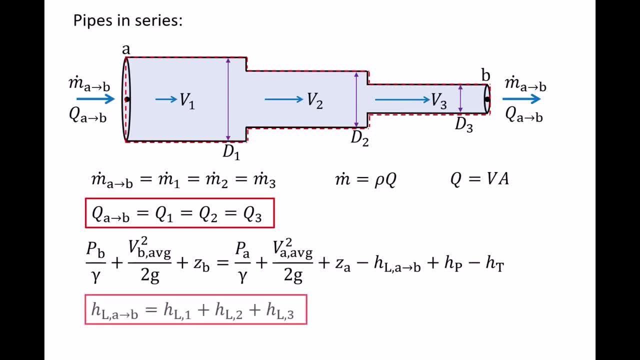 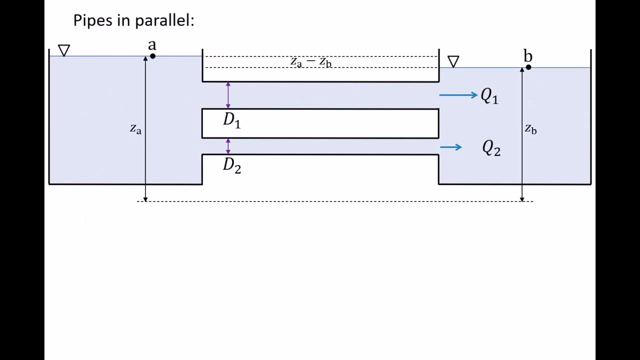 Since the flow must travel through all three pipes, the total head loss is simply the sum of the head loss through each of the three pipes. Now let's look at a system where the flow can travel through pipes in parallel. Here we have two water reservoirs connected by two pipes. 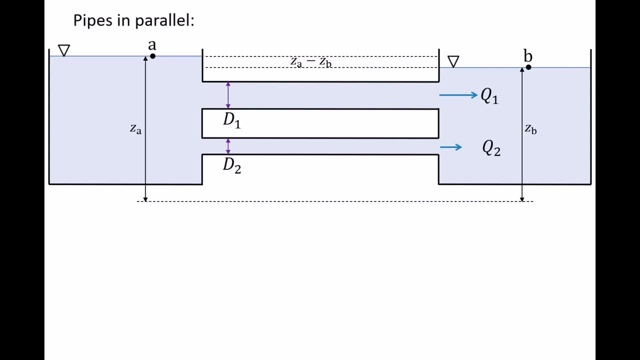 The reservoir on the left has a free surface at point A and the reservoir on the right has a free surface at point B. We will assume the elevation difference ZA minus ZB is known. Since free surface A is at a higher elevation compared to free surface B, water will flow. 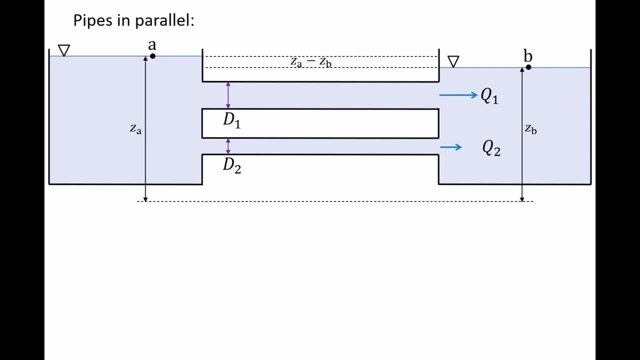 from the left reservoir to the right reservoir, A volumetric flow rate- Q1,- flows through pipe 1 and a volumetric flow rate Q2, flows through pipe 2.. The total volumetric flow rate from reservoir A to reservoir B- QAB- is the sum of the flow. 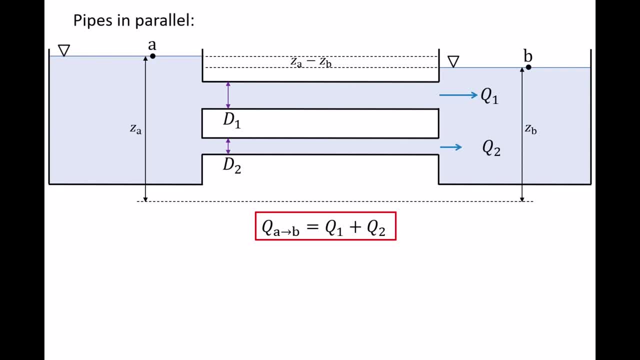 rates through both pipes, Q1 plus Q2.. If the pipe diameters D1 and D2 are different, the speeds V1 and V2 and flow rates Q1 and Q2 will differ. Now we will determine the relationship between the head loss in pipe 1 and the head loss. 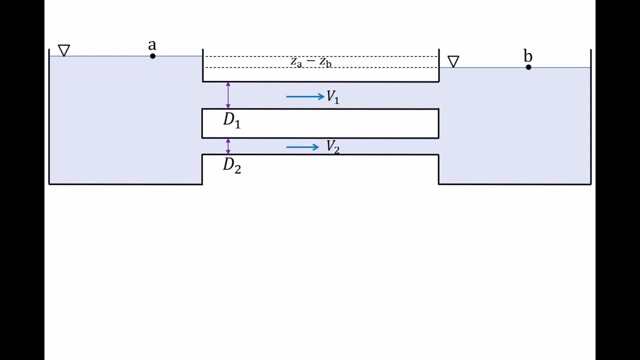 in pipe 2.. We assume the reservoirs are so large that the elevation doesn't change significantly over the time period. we observe them. Since a constant head is applied at the inlet and outlet of each pipe, this means the flow through each pipe is constant in time. 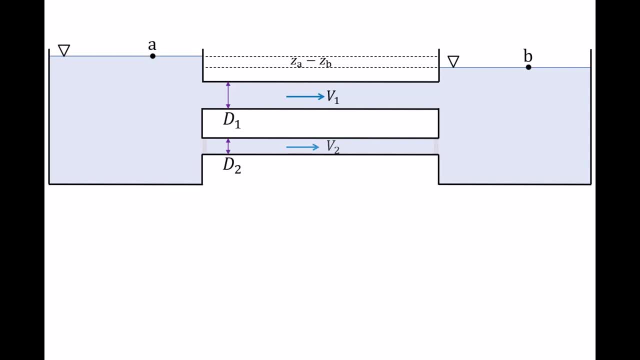 This also means that the flow through each pipe is independent and we can plug up pipe 2 without it impacting the flow. This means that the flow through each pipe is constant in time. Now that the flow through pipe 1 is isolated, we draw a control volume with an inlet at 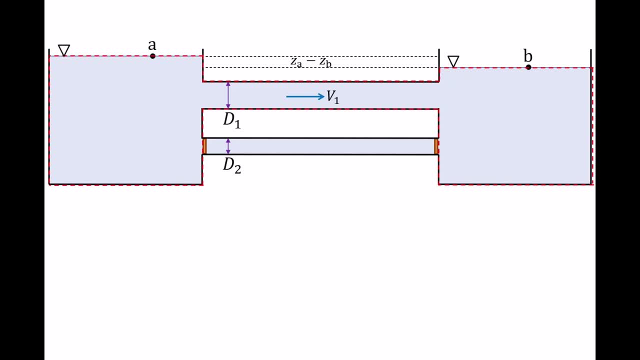 free surface A and an outlet at free surface B. The conservation of energy equation is the pressure head plus velocity head plus elevation head at B. equals the pressure head plus velocity head plus elevation head at A, minus the head loss related to the flow through pipe 1, HL1, plus the pump head minus the turbine head. 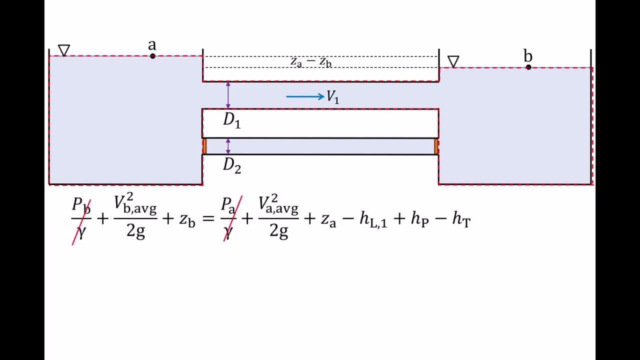 The pressure difference between free surface A and free surface B is usually negligible compared to the other terms in the equation, so we eliminate the pressure heads. Since points A and B are at the top of the reservoirs and the water level does not change significantly in time, the speed at those points is zero, which means the velocity head. 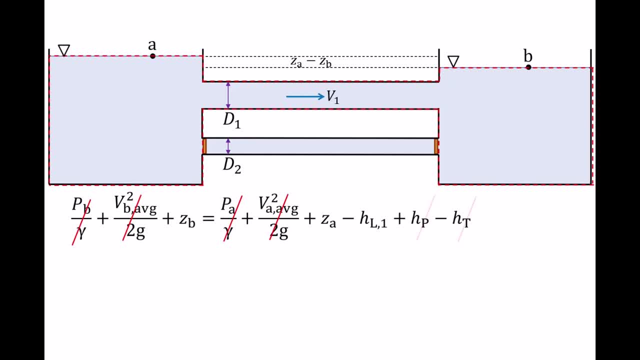 terms are zero too. The pump head and turbine head are zero because no pumps or turbines exist in the control volume. Rearrangement, Rearranging the remaining terms, gives us that the difference in elevation heads, ZA minus ZB, is equal to the head loss HL1.. 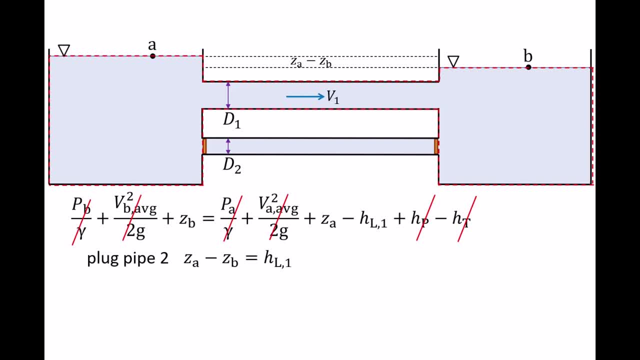 This means the head loss through pipe 1 is only related to the difference in elevation of the free surfaces, which is constant. Now notice: our decision to plug up pipe 2 was arbitrary. If we plugged up pipe 1 and analyzed the flow through pipe 2 instead, we would find that 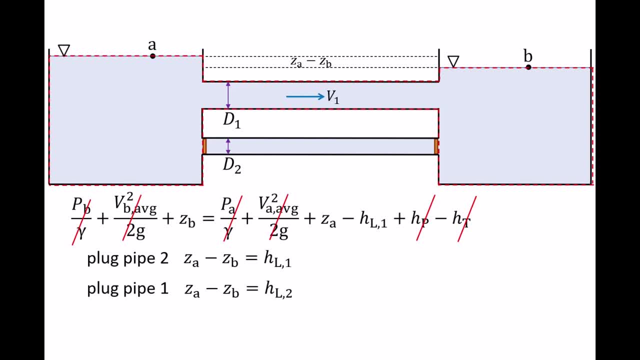 ZA minus ZB is equal to HL2.. So we plug up pipe 1 and analyze the flow through pipe 2 instead. we would find that ZA minus ZB is equal to HL2.. So for a parallel pipe configuration, the head losses through the pipes are equal. 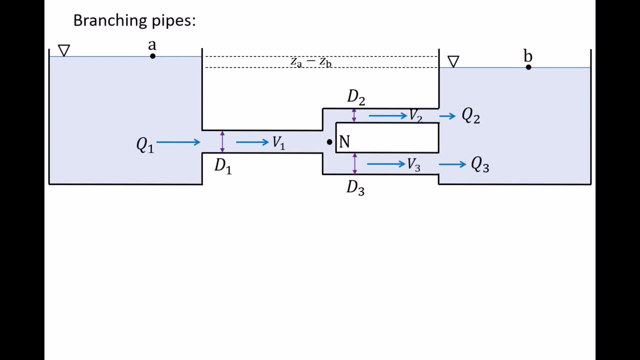 The last system that we'll examine has pipes that branch or split at a node N. We'll keep the same reservoirs A and B but connect them with a different set of pipes. Reservoir A is connected to pipe 1, and the entire flow Q1, must travel through this. 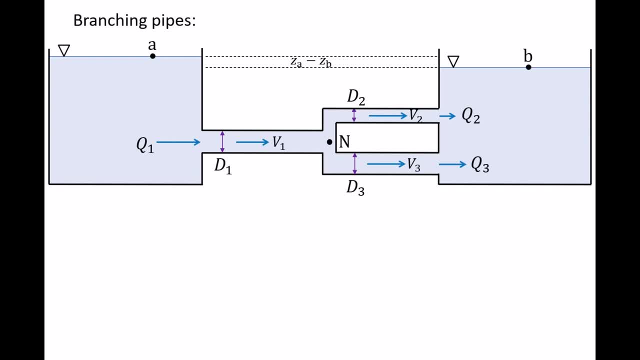 pipe to node N. At the node, the flow can travel through pipe 2 or pipe 3 to enter reservoir B. The flow rate through pipe 2 is Q2, and the flow rate through pipe 3 is Q3.. Since the entire flow from reservoir A to reservoir B must travel through pipe 1, and 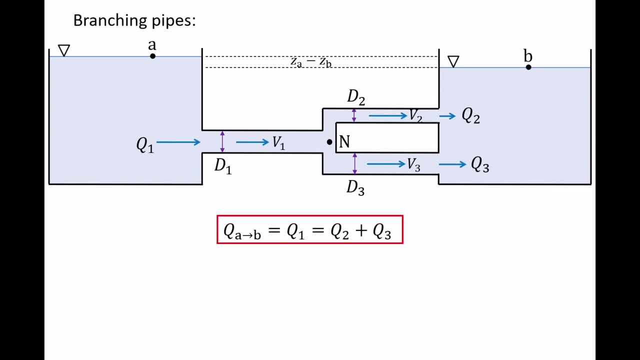 then the entire flow must travel through either pipe 2 or pipe 3, the total volumetric flow rate, QAB, is equal to Q1, which is also equal to the sum of Q2 plus Q3.. If we isolate the node with a control volume, we see that the water flows into the control. 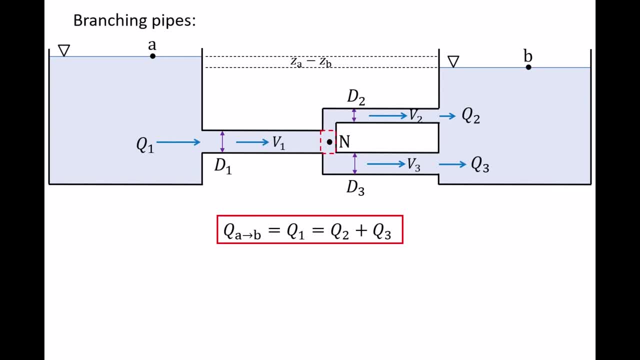 volume from pipe 1 and flows out of the control volume through pipe 2 and pipe 3.. There's one inlet and two outlets for this control volume. We can generalize the conservation of mass equation for a case where there may be multiple inlets and outlets. 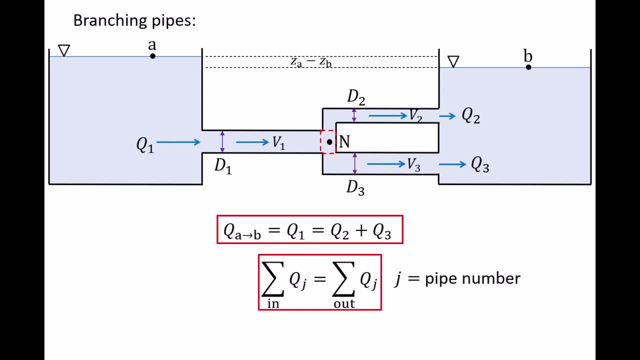 The sum of all volumetric flow rates into a node is equal to the sum of all volumetric flow rates out of a node, Where here we have replaced the pipe number with the index j. Now we will determine the relationship between the head losses in the branching pipes. 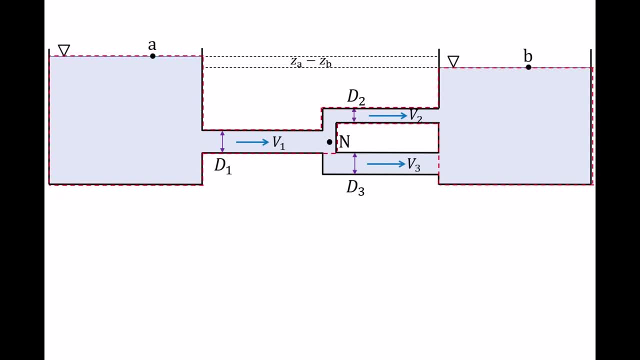 We draw a control volume for the fluid that travels through pipe 1 and the top branch pipe 2.. The inlet of the control volume is at free surface A and the outlet is at free surface B. The conservation of energy equation is the pressure head plus velocity, head plus elevation.